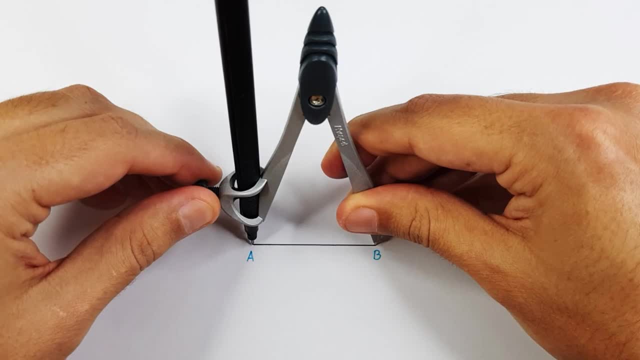 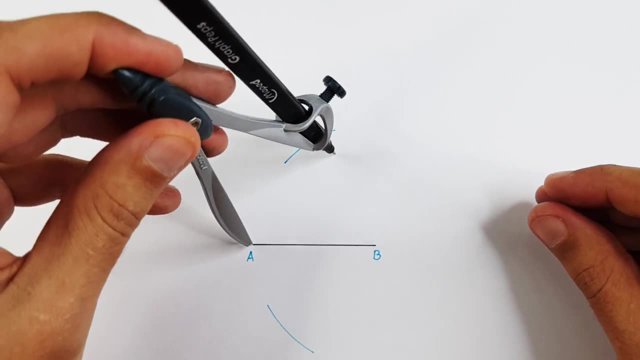 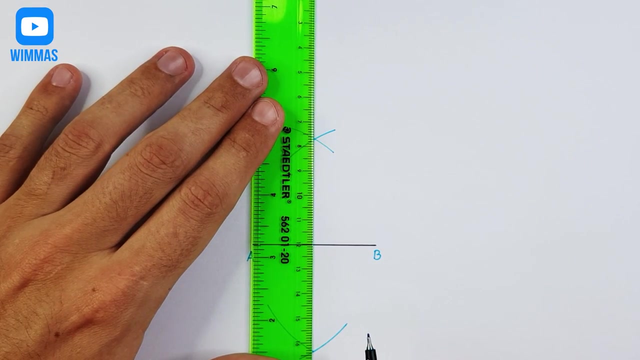 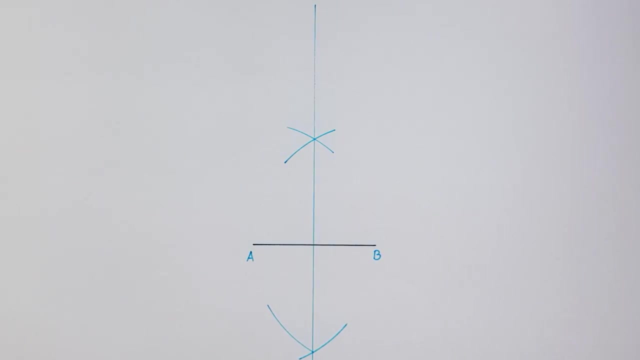 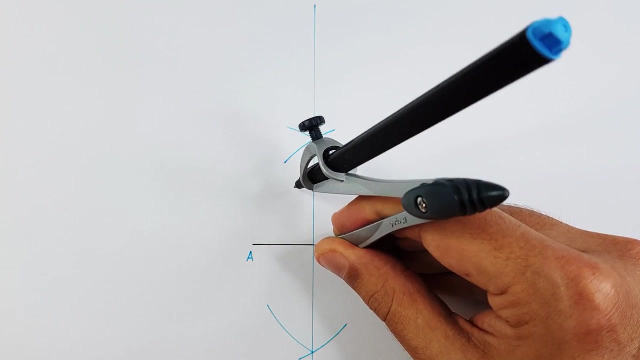 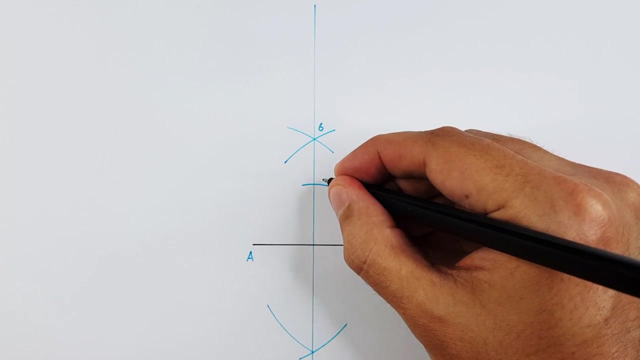 Start off by taking your compass and applying the middle point method using the full length of the line. Place your compass on the middle point and project point A onto your middle point method. The top intersection can be labeled as 6 and the second one can be labeled as 4.. 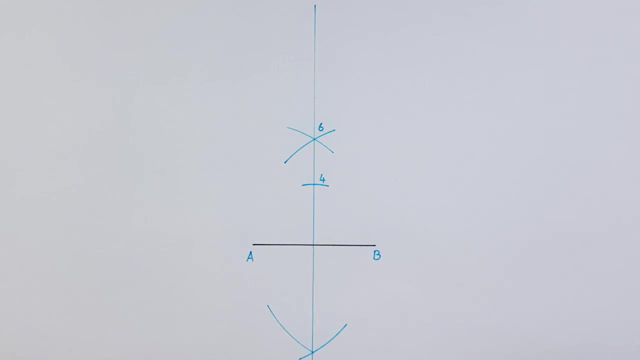 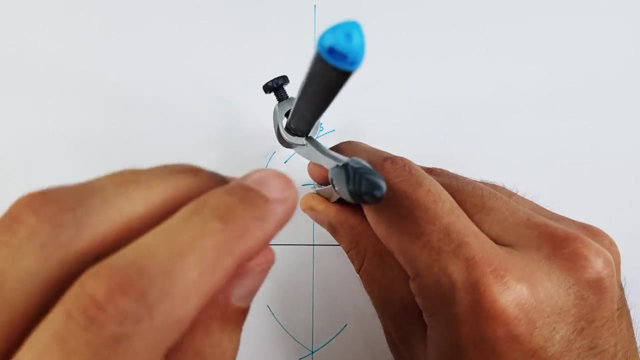 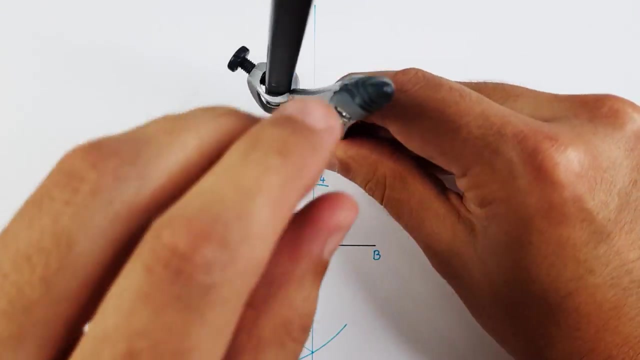 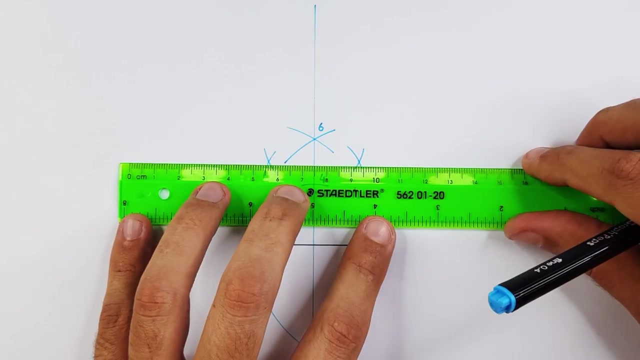 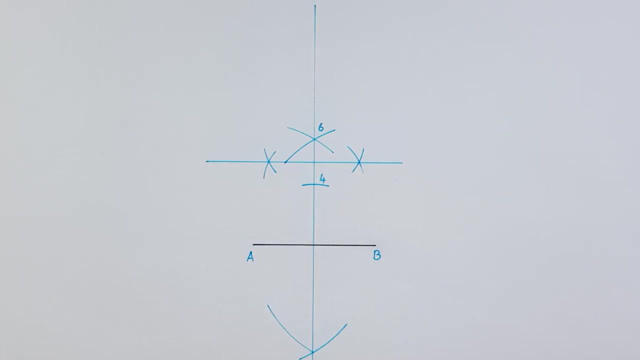 To draw a pentagon, we need to determine point 5.. To do that, we need to determine the middle point between point 6 and 4.. So it's very simple: Apply the middle point method between point 6 and 4.. Once you have determined the middle point, label it as point 5.. 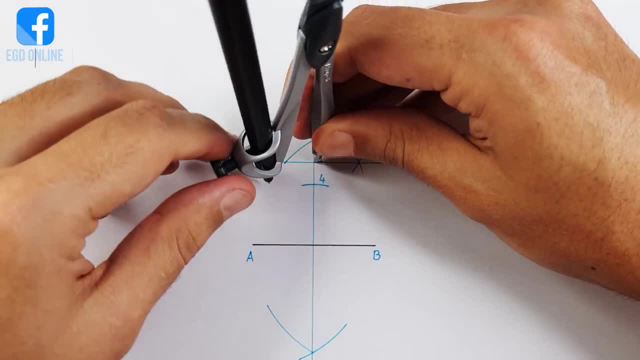 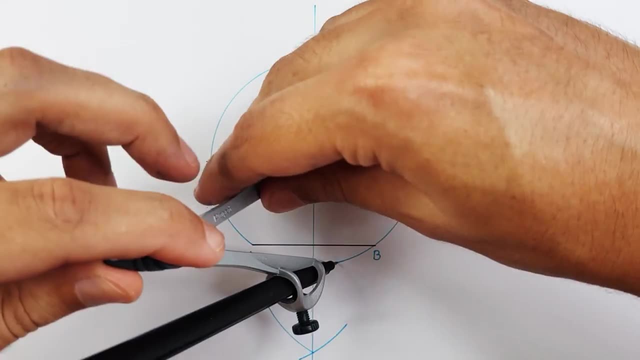 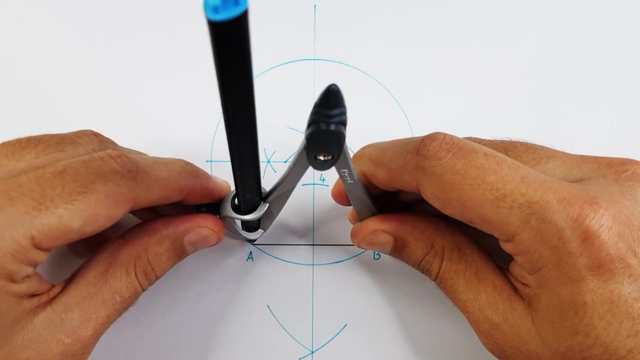 Place your compass on point 5 and adjust it to point A. Draw the circle that we will need to draw. In this case it is 7 inches. We're going to use our compass to determine our pentagon. We can then use our compass and take the full side length and determine our pentagon on our circle. 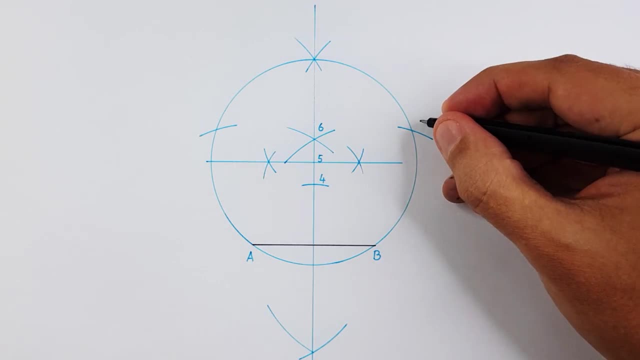 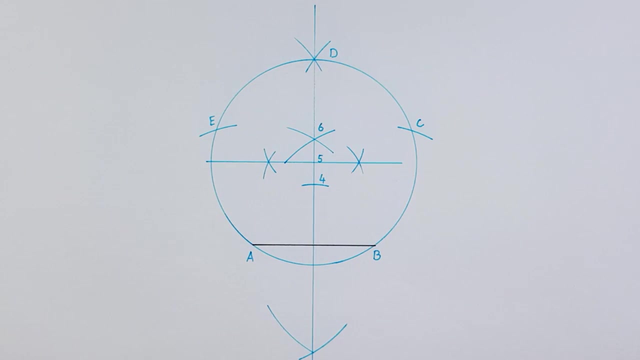 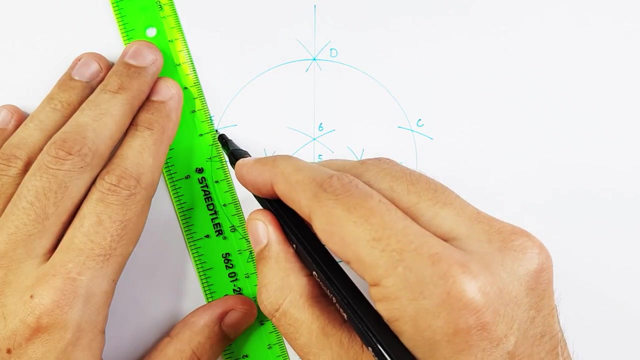 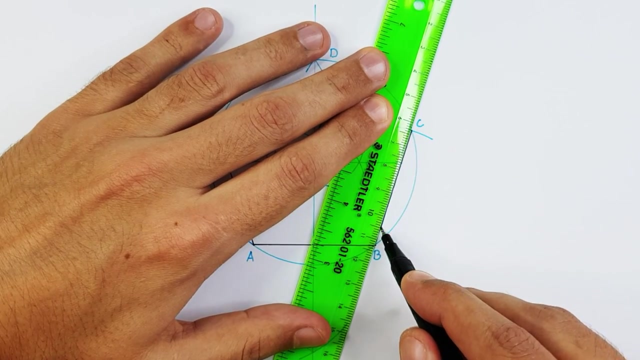 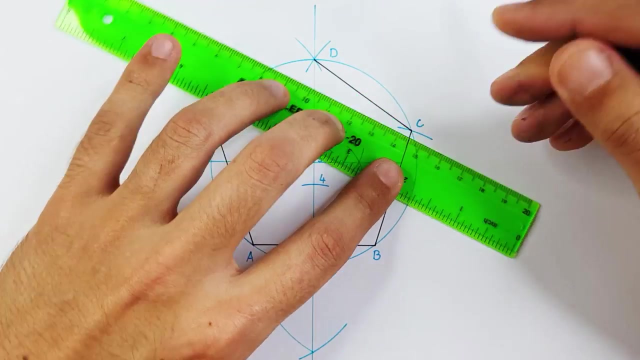 You can label these points as point C, 3 and 6.. You can label these points as points C, D and E. For the final step, take your ruler and draw your pentagon. If you found this method helpful, don't forget to like the video and also to subscribe to the channel. 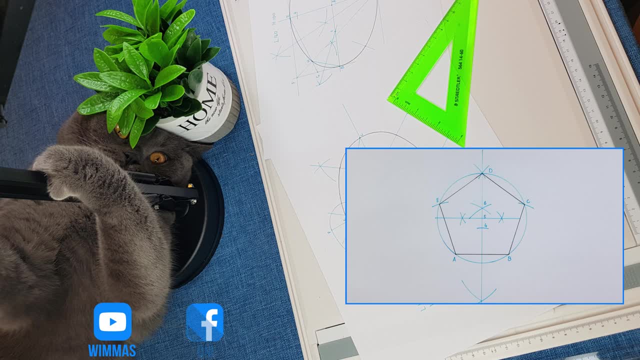 Also, don't forget to have a look at some of the other videos I have on this channel. But until then, I'll catch you in the next one.